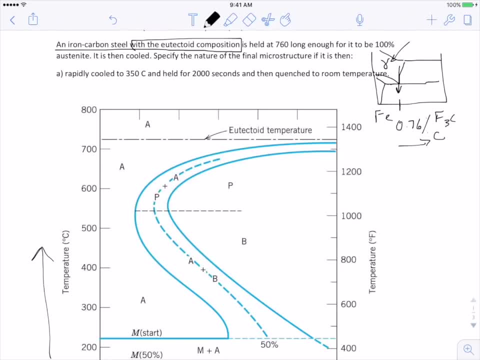 of 0.76 weight percent carbon. This is composition on that axis. So a eutectoid composition steel means it has 0.76 weight percent carbon and that all of it is going to form pearlite as a. it goes on through that temperature. Again, this is review. The eutectoid reaction refers to austenite. 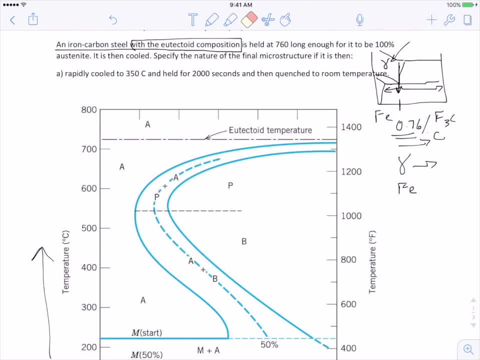 going to make ferrite. Excuse me, I'm going to rewrite that Ferrite is given the symbol alpha plus Fe3C. So that is the eutectoid reaction. All right, so that's all stuff you kind of need to know already from the. 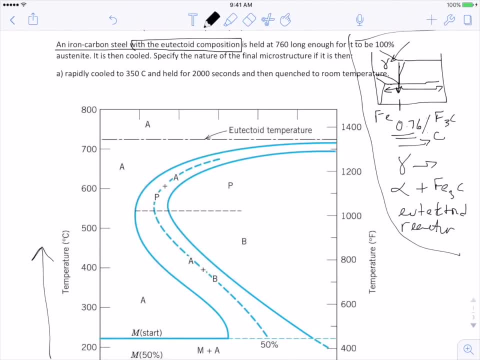 previous chapter, but I'm just putting it back in your head Now again, from the previous eutectoid reaction, which occurs at 7.27.. So now, looking at this T-j bomb and labeled the eutectoid temperature, 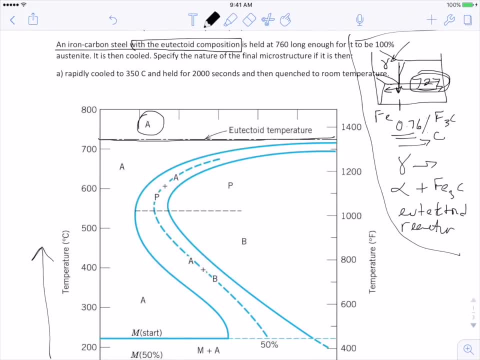 notice that above the eutectoid temperature there's an A. A stands for austenite right. That is because that is the stable phase that exists for eutectoid steel above that temperature. Now the equilibrium phase is that the minute we go below 7.27,. 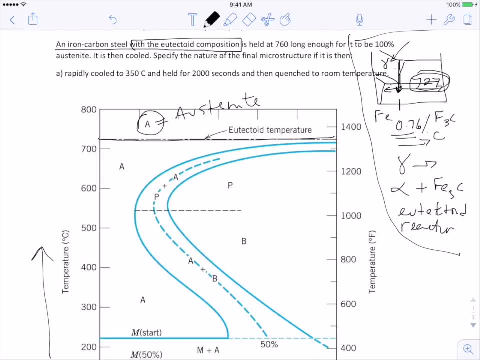 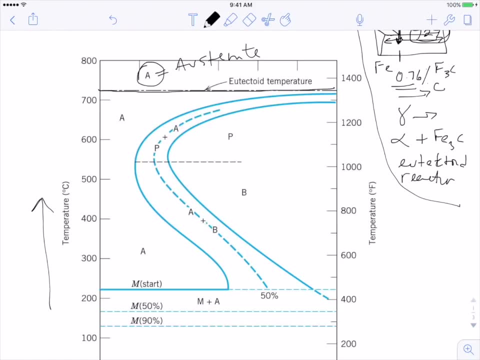 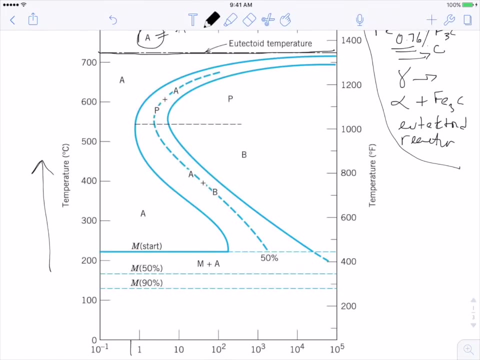 austenite ceases to exist and that it turns into perlite. But this diagram, this TT, if we, for example, take this steel and we quench it, that means rapidly cool. and if we cool it in less than a second, for example. 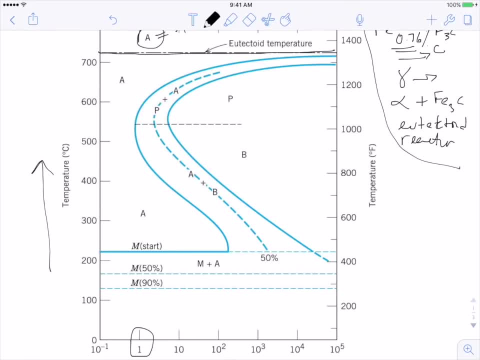 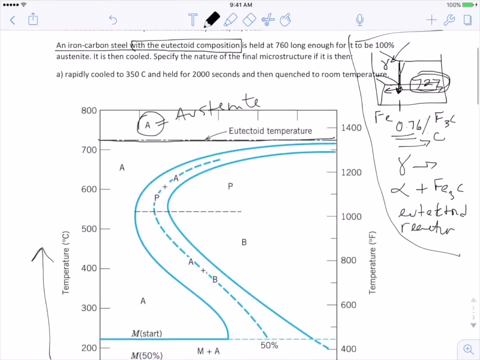 down to room temperature. it turns out that the transformation happens too fast for any perlite to form, And then in that case we would end up with martensite forming, and we'll talk more about that later. So let's just kind of go through what it's: we're: cooling it to 350,. 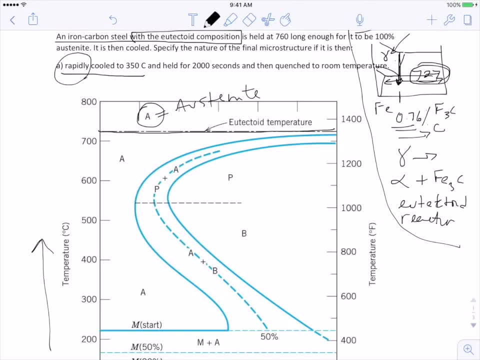 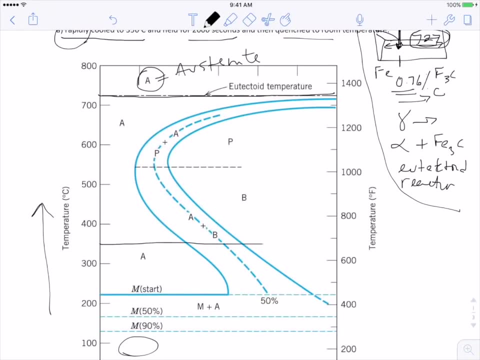 and so you can use the word rapidly as meaning kind of instantly, and held for 2,000 seconds, and then it's quenched to room temperature. Draw a horizontal line just to orient myself. So and we've been told it's rapidly cooled. so let's imagine it happens pretty darn fast. 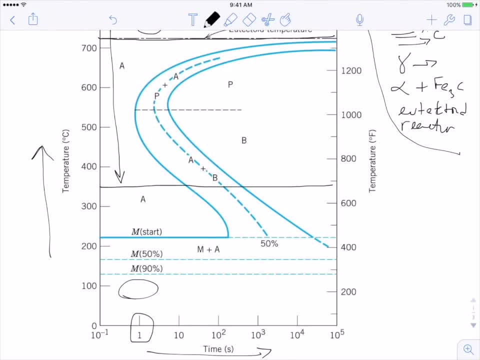 and then we're going to cool it down. We're holding it in place for 2,000 seconds, so I have access 10 to the third is, of course, 1,000, so 2,000 seconds might be approximately there, so I'm going to look.